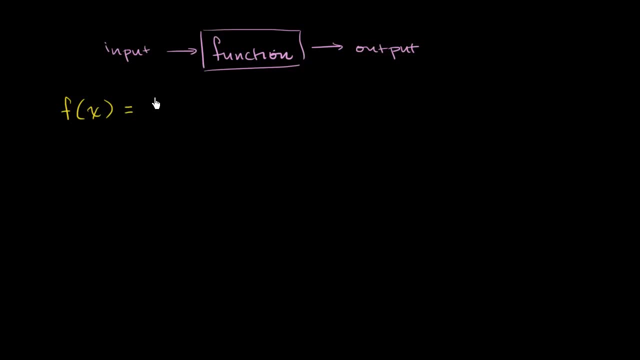 but we'll see that you can use others. But we could have: f of x is equal to is equal to, let's say, x squared if x is even. and let's say it is equal to x plus 5, if x is. 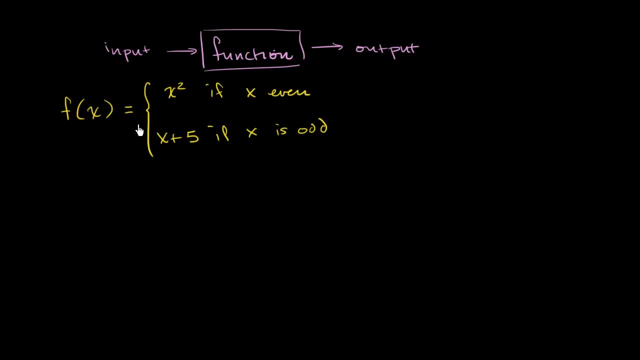 if x is odd. So what would happen if we input 2 into this function And the way that we would denote inputting 2 is that we would want to evaluate f of 2.. This is saying, let's input 2 into our function, f. 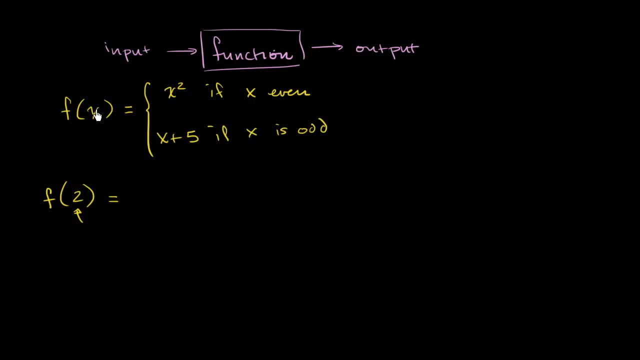 And everywhere we see this x, here, this variable. you can kind of use this as a placeholder. let's replace it with our input. So let's see: if 2 is even, do 2 squared. if 2 is odd, do 2 plus 5.. 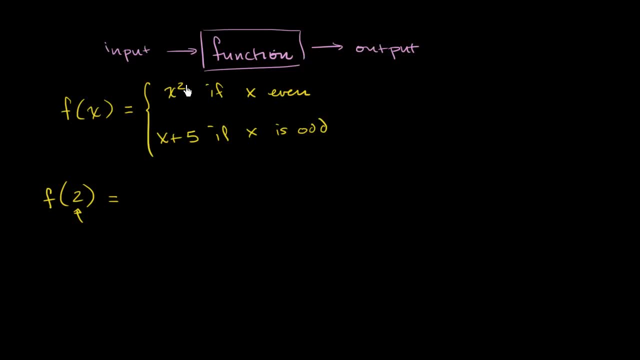 Well, 2 is even so, we're going to do 2 squared. So in this case, f of 2 is going to be 2 squared or 4.. Now, what would f of f of 3 be? 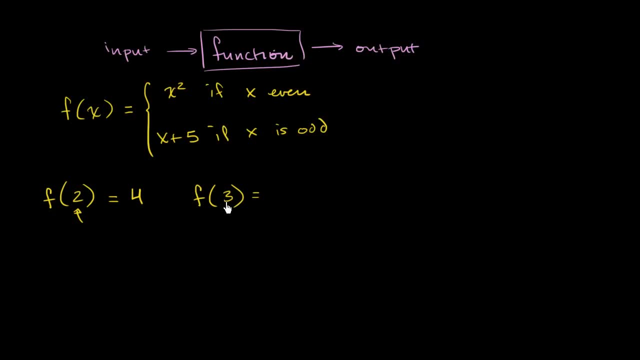 Well, once again, everywhere we see this variable, we'll replace it with our input. We'll replace it with our input. So f of 3, so 3 squared if 3 is even 3 plus 5 if 3 is odd. 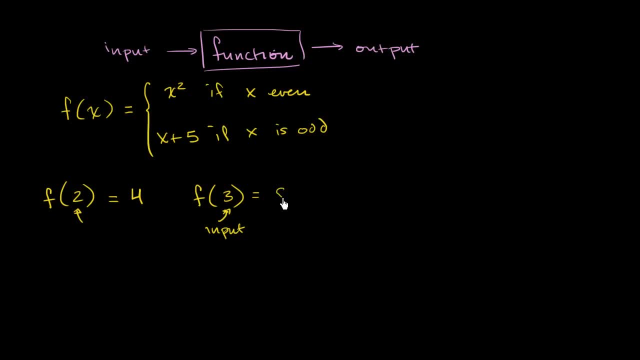 Well, 3 is odd, so it's going to be 3 plus 5, it is going to be equal to 8.. Now you might say: okay, that's neat, Sal. This was kind of an interesting way to define a function. 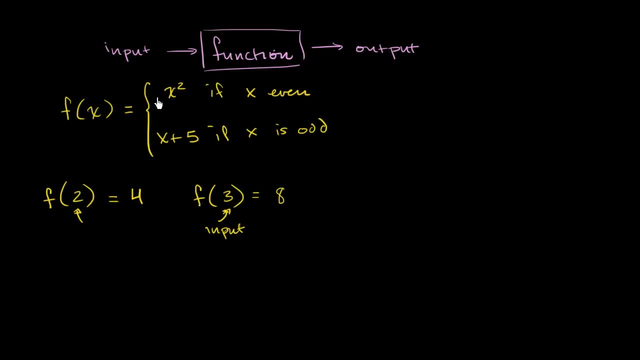 a way to kind of munch on these numbers. But you know, I could have done this with traditional equations in some way, especially if you allowed me to use the squirrely bracket thing. What can a function do that maybe my traditional tool kits might have not been as expressive about? 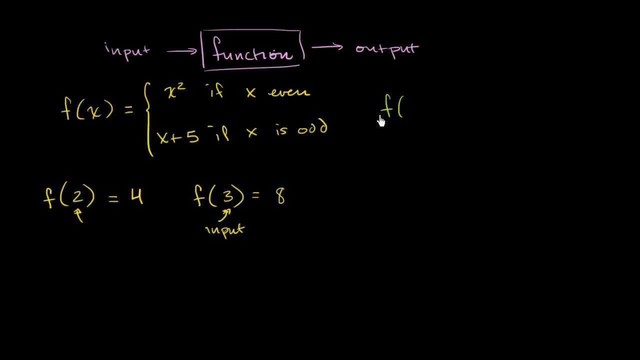 Well, you could even do a function like this. You could have it. Let me not use f and x anymore, just to show you that the notation is more general than that. So I could say: h of a is equal to, is equal to the next largest number. 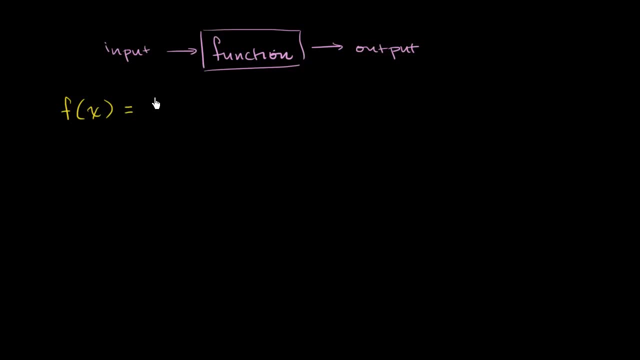 but we'll see that you can use others. But we could have: f of x is equal to is equal to, let's say, x squared if x is even. and let's say it is equal to x plus 5, if x is. 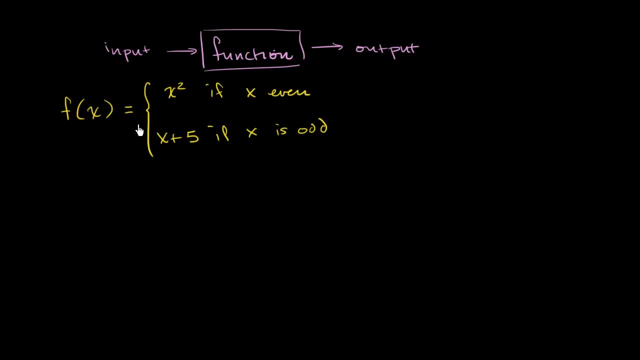 if x is odd. So what would happen if we input 2 into this function And the way that we would denote inputting 2 is that we would want to evaluate f of 2.. This is saying, let's input 2 into our function, f. 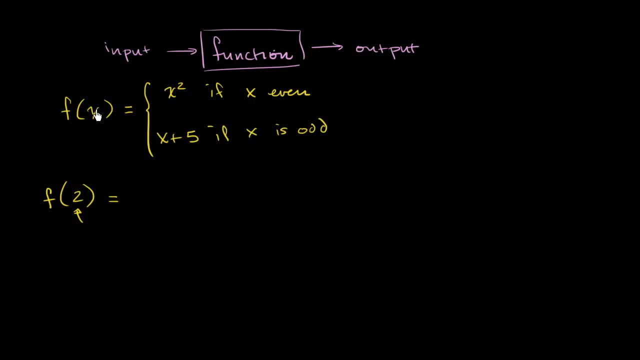 And everywhere we see this x, here, this variable. you can kind of use this as a placeholder. let's replace it with our input. So let's see: if 2 is even, do 2 squared. if 2 is odd, do 2 plus 5.. 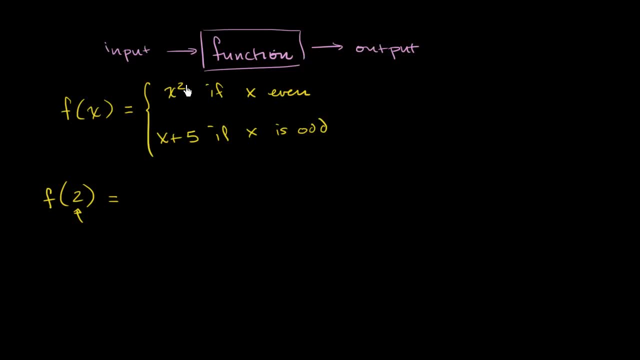 Well, 2 is even so, we're going to do 2 squared. So in this case, f of 2 is going to be 2 squared or 4.. Now, what would f of f of 3 be? 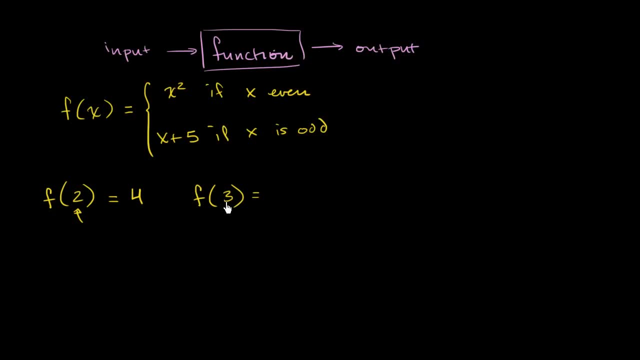 Well, once again, everywhere we see this variable, we'll replace it with our input. We'll replace it with our input. So f of 3, so 3 squared if 3 is even 3 plus 5 if 3 is odd. 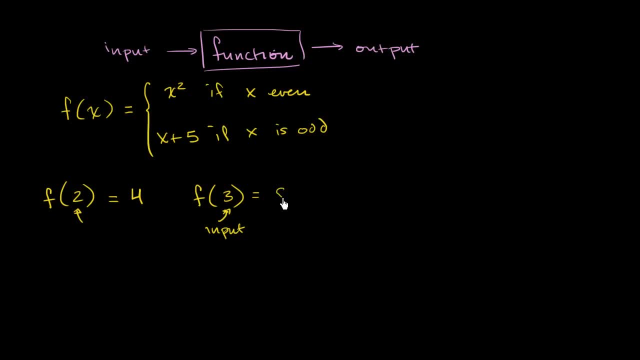 Well, 3 is odd, so it's going to be 3 plus 5, it is going to be equal to 8.. Now you might say: okay, that's neat, Sal. This was kind of an interesting way to define a function. 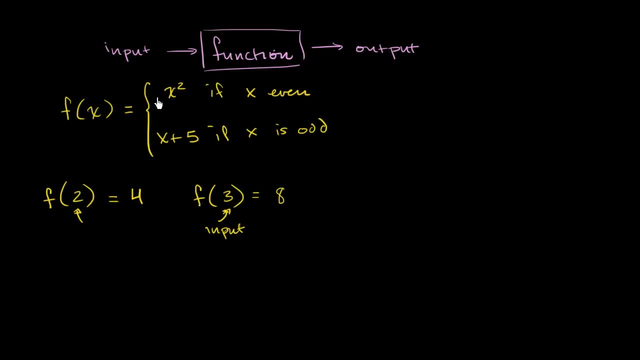 a way to kind of munch on these numbers. But you know, I could have done this with traditional equations in some way, especially if you allowed me to use the squirrely bracket thing. What can a function do that maybe my traditional tool kits might have not been as expressive about? 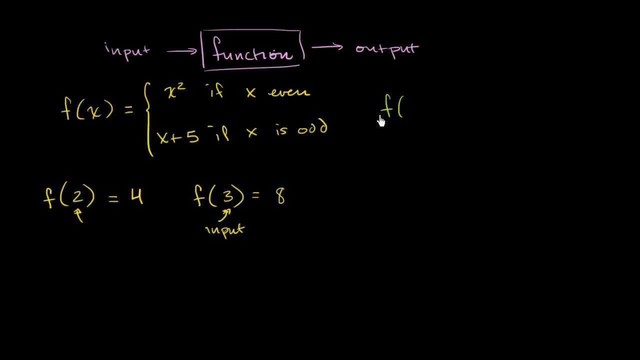 Well, you could even do a function like this. You could have it. Let me not use f and x anymore, just to show you that the notation is more general than that. So I could say: h of a is equal to, is equal to the next largest number. 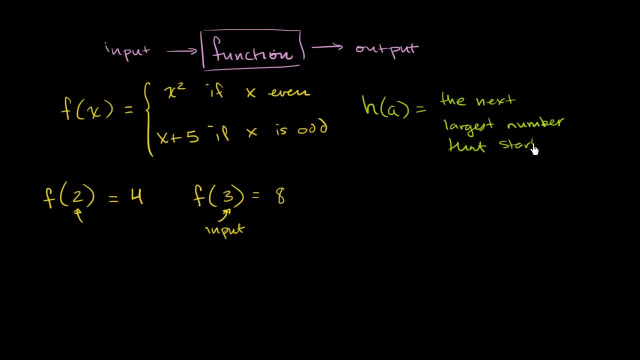 that starts with the same letter. the same letter, letter as variable a. it says as variable a and we're going to assume that we are dealing in English. So, given that, what is h of what is h of 2 going to be? 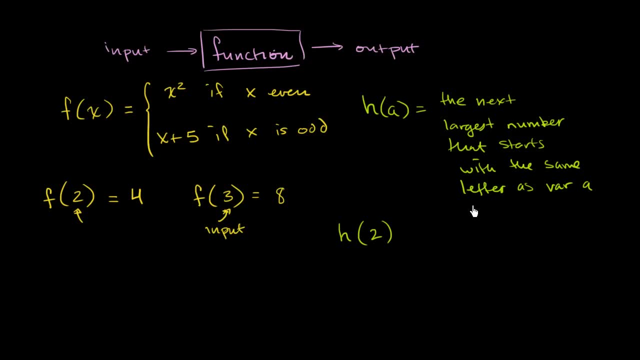 Well, 2 starts with a t. What's the next largest number that starts with a t? Well, it's going to be. it's going to be equal to 3.. Now, what would h of? I don't know. let's think about this. 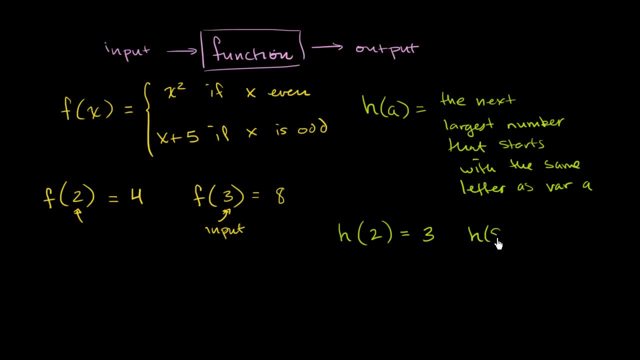 What would h of h of 8 be equal to? Well, 8 starts with an e, The next largest number that starts with an e. so it's not 9,, 10,, it would be. it would be 11.. 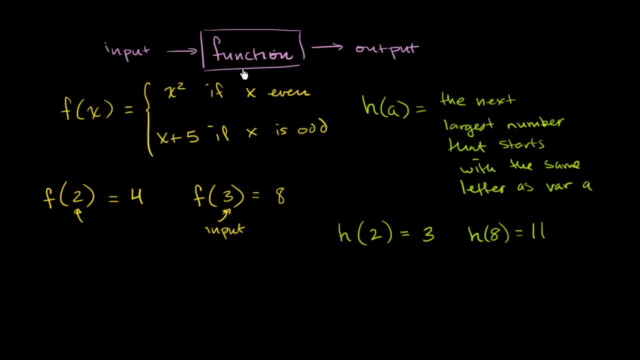 And so now you see, it's a very, very, very general tool. This function is this h function that we just defined. we'll look at it. we'll look at the letter that the number starts with in English. so it's doing this really really, really, really wacky thing. 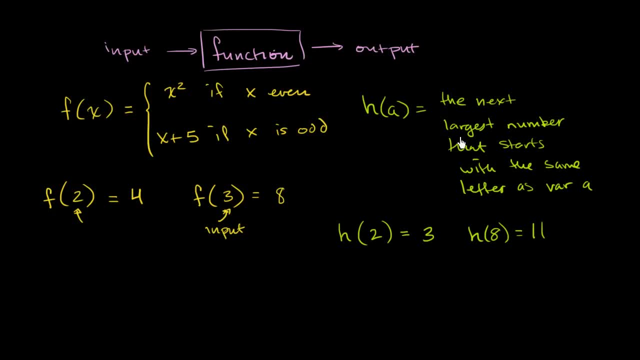 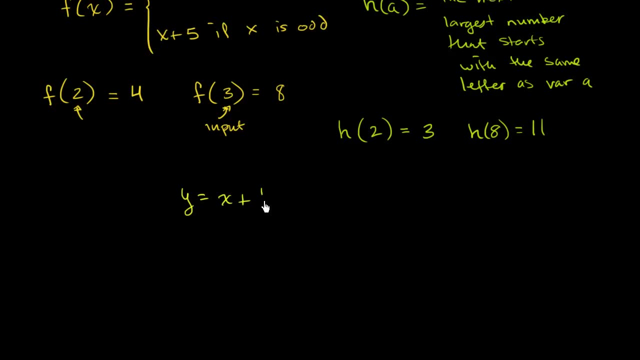 Now, not all functions have to be this wacky. In fact, you have already been dealing with functions. You have seen things like. you have seen things like: y is equal to x plus 1. This can be viewed as a function. 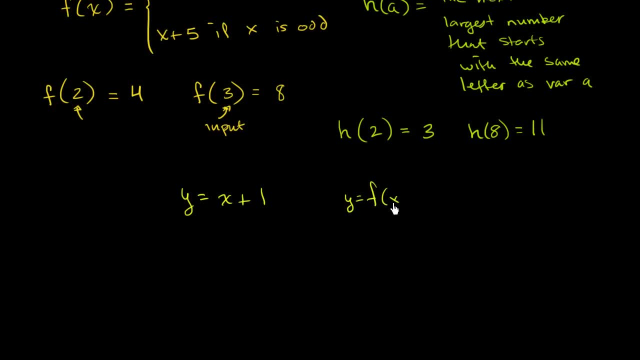 We could write this as: y is a function of x, which is equal to x plus 1.. If you give as an input, as you give as an input, so let me write it this way. So, for example, when we could: 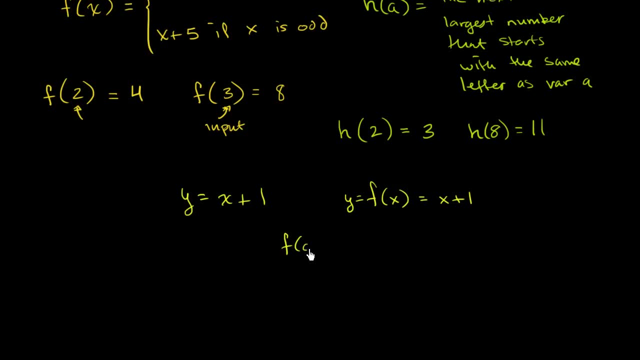 when x is 0, we could say f of 0, f of 0 is equal to well, you take 0,, you add 1, it's equal to 1.. f of 2 is equal to 2.. 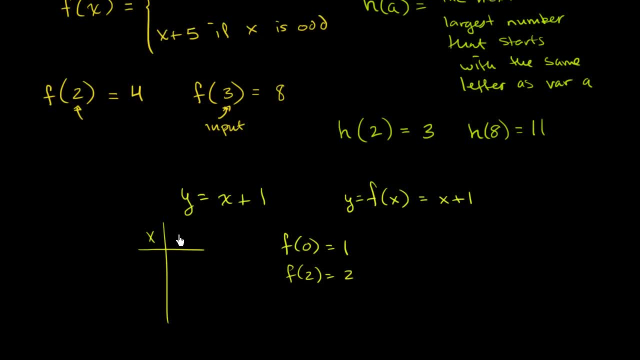 You've already done this before. You've done things where you said: look, let me make a table of x, Let me take and put our y's there. When x is 0, y is 1.. When x is 2,. I'm sorry. 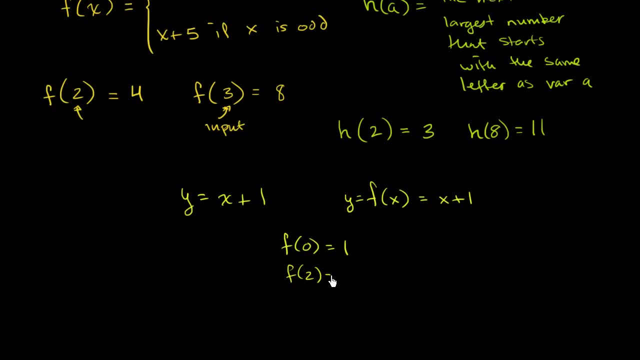 this was when x is, I made a little mistake where f of 2 is equal to 3.. And you've done this before with tables where you say: look x and y, when x is 0, y is 1.. 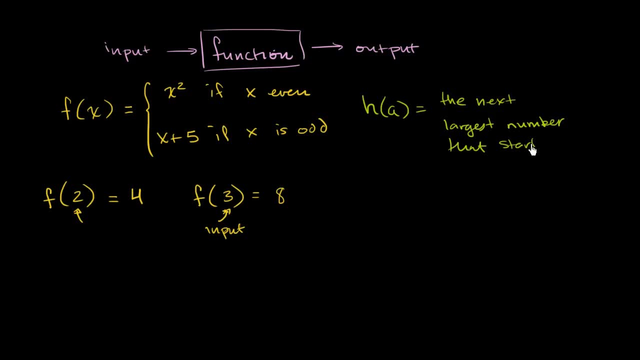 that starts with the same letter. the same letter, letter as variable a. It says as variable a, And we're going to assume that we are dealing in English. So, given that, what is h of 2 going to be? Well, 2 starts with a, t. 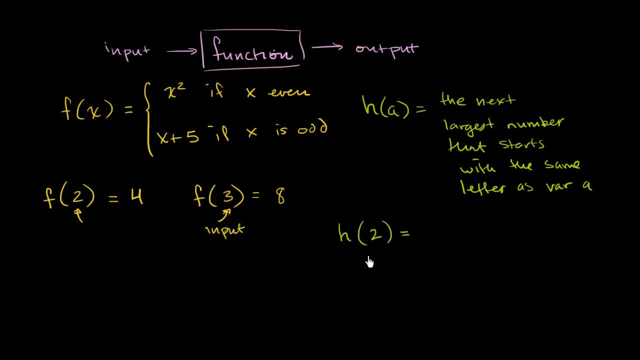 What's the next largest number that starts with a, t? Well, it's going to be. it's going to be equal to 3.. Now, what would h of? I don't know. let's think about this. What would h of h of 8 be equal to? 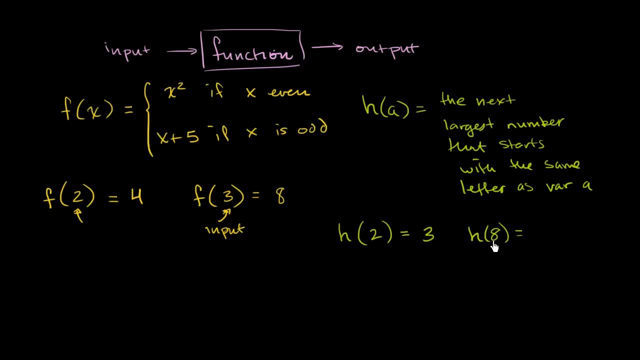 Well, 8 starts with an e, The next largest number that starts with an e. so it's not 9,, 10, it would be, it would be 11.. And so now you see, it's a very, very, very general tool. 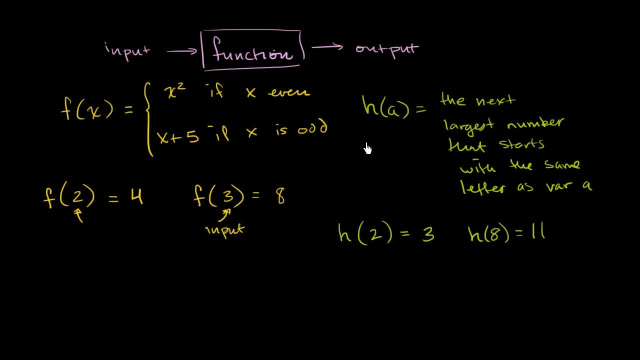 This function is this h function that we just defined. we'll look at it. we'll look at the letter that the number starts with in English. So it's doing this really, really, really, really wacky thing. Now, not all functions have to be this wacky. 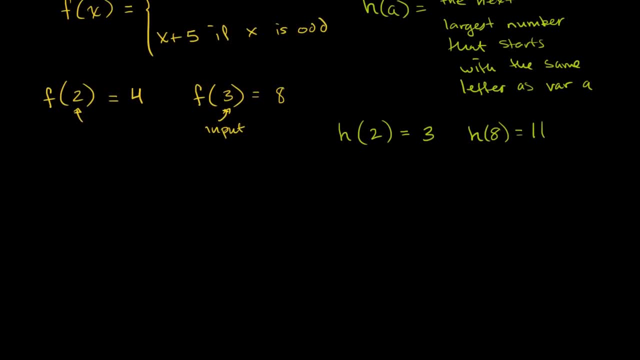 In fact, you have already been dealing with functions. You have seen things like. you have seen things like: y is equal to x plus 1.. This can be viewed as a function. We could write this as: y is a function of x, which is equal to x plus 1.. 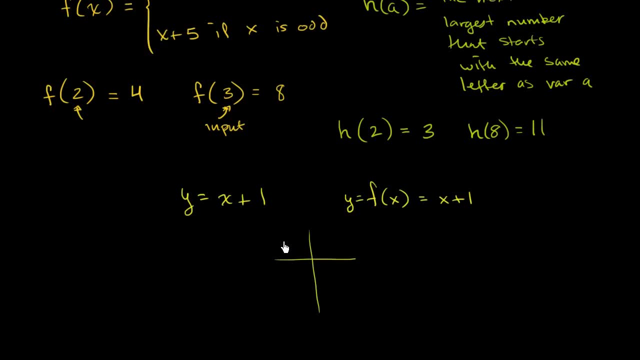 If you give as an input, as you give as an input. so let me write it this way. So, for example, when we could, when x is 0, we could say: f of 0 is equal to well, you take 0,, you add 1,, it's equal to 1.. 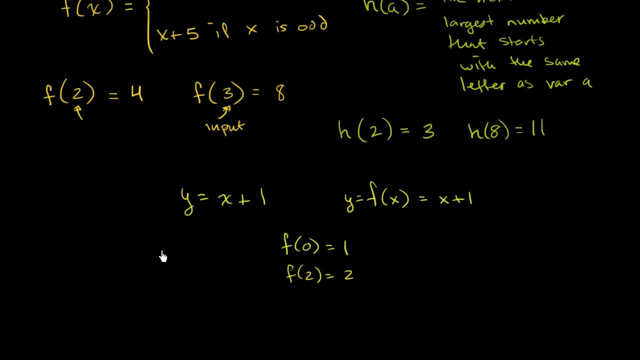 f of 2 is equal to 2.. You've already done this before. You've done things where you said: look, let me make a table of x, Let me take and put our y's there When x is 0, y is 1.. 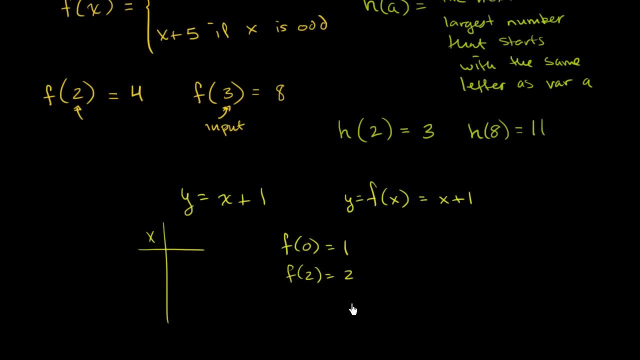 When x is 2, I'm sorry, this was when x is. I made a little mistake where f of 2 is equal to 3.. And you've done this before with tables where you say: look x and y, when x is 0, y is 1.. 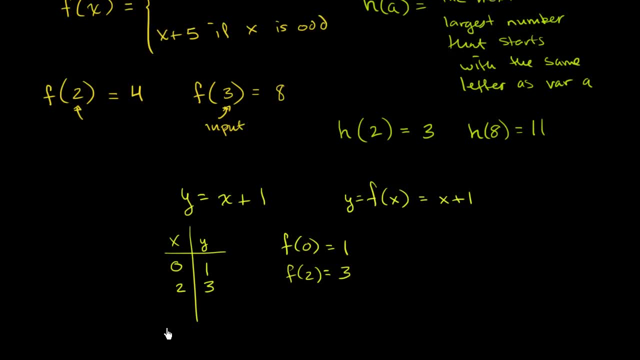 When x is 2, y is 3.. So this you might say: well, what was the whole point of using the function notation here to say f of x is equal to x plus 1? And the whole point is to think: 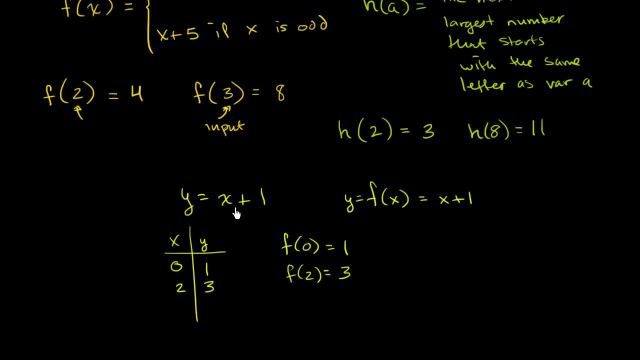 in these more general terms. For something like this you didn't really have to introduce function notations. but it doesn't hurt to introduce function notations because it makes it very clear that a function takes an input. takes my x and this definition. 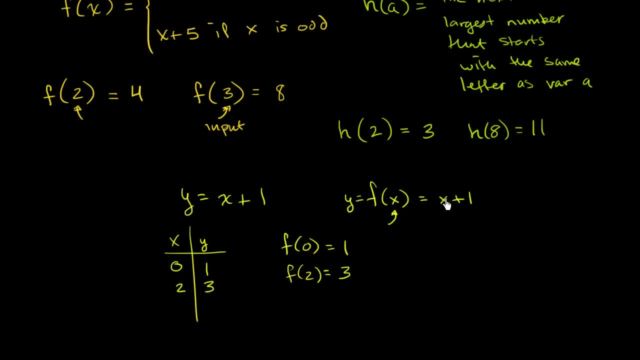 it munches, it munches on it, it says okay, x plus 1, and then it produces one more than it. So here, whatever the input is, the output is one more than that original function. Now I know what you're asking. 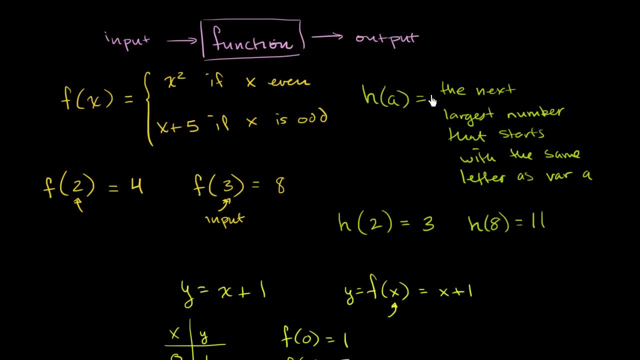 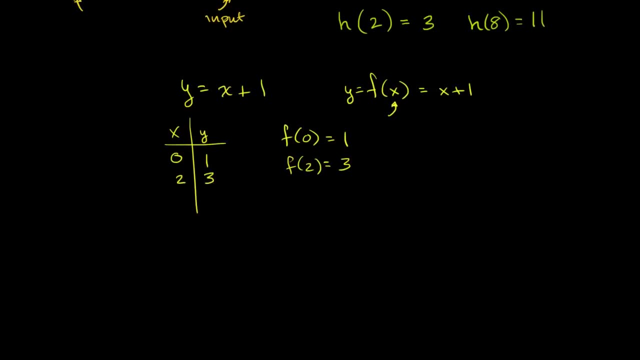 All right. Well, what is not a function then? Well, remember, we said: a function is something that takes an input and produces only one possible output for that given input. So, for example, something like- and let me look at a visual way: 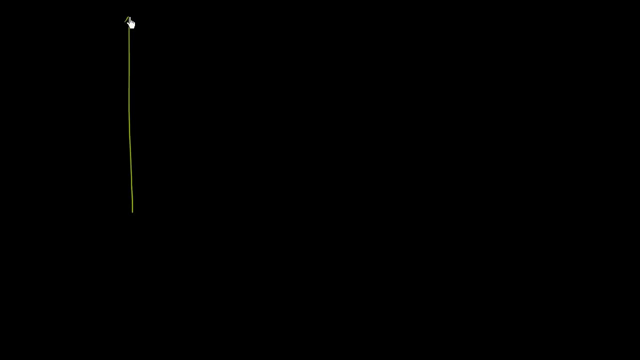 of thinking about a function this time, or a relationship, I should say So. let's say that's our y-axis and this right over here is our x-axis. And let me draw a circle here. that has radius. let me draw a circle here. 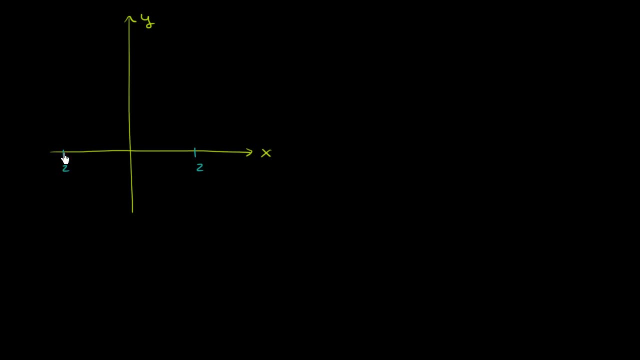 that has radius 2.. So it's a circle of radius 2.. This is negative, 2.. This is positive, 2.. This is negative, 2.. So my circle, it's centered at the origin. It has radius 2,. 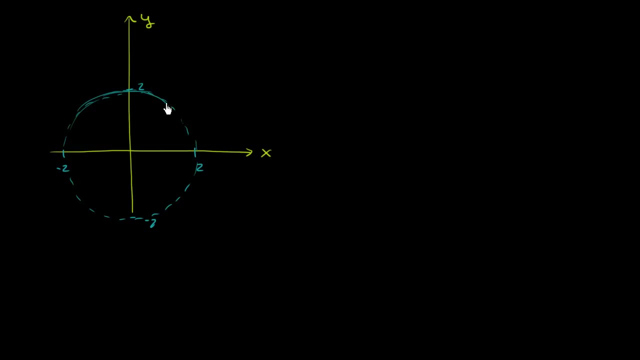 so that's my best attempt at drawing the circle. Let me fill it in. So this is a circle. The equation of a circle, of this circle, is going to be: x squared plus y squared is equal to the radius squared is equal to 2 squared. 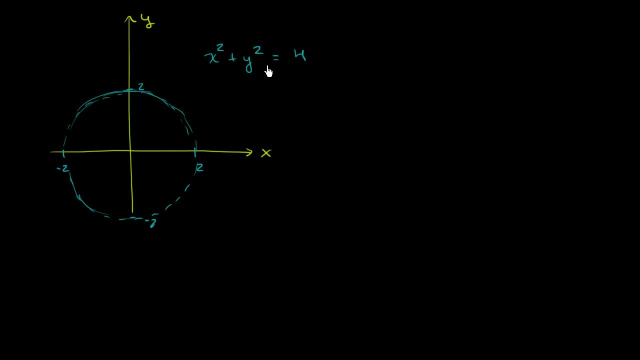 or it's equal to 4.. So the question is: is this relationship between x and y? here I've expressed it as equation, here I've visually drawn all of the x's and y's that satisfy this equation. Is this relationship between x and y? 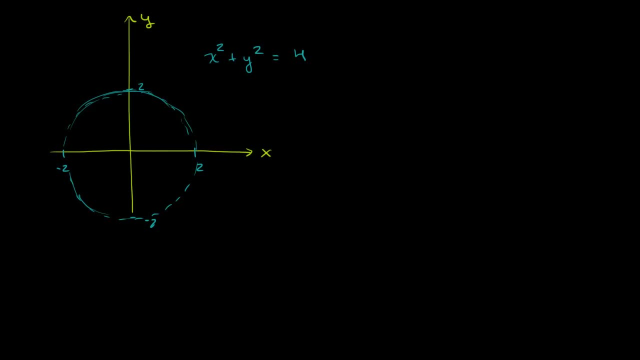 a function And we can see visually that it's not going to be a function. You pick a given x. Let's say x is equal to 1.. Let's say x is equal to 1.. There's two possible y's that are associated with it. 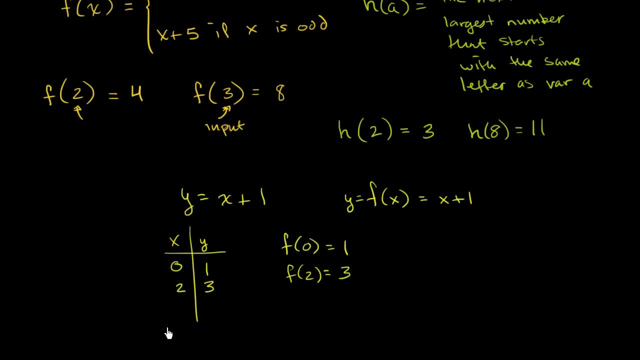 When x is 2, y is 3.. So this you might say: well, what was the whole point of using the function notation here to say f of x is equal to x plus 1?? And the whole point is to think in these more general terms. 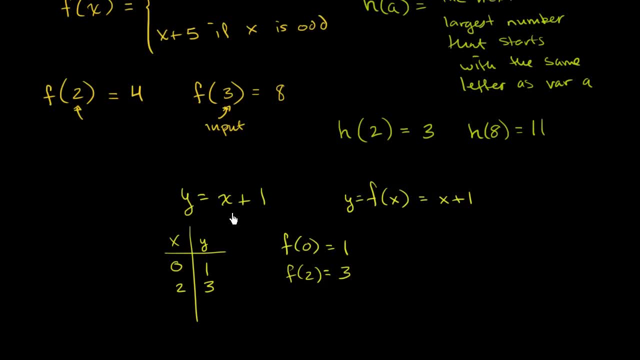 For something like this you didn't really have to introduce function notations. but it doesn't hurt to introduce function notations because it makes it very clear that a function takes an input. takes my x and this definition, it munches on it. it says okay, x plus 1,. 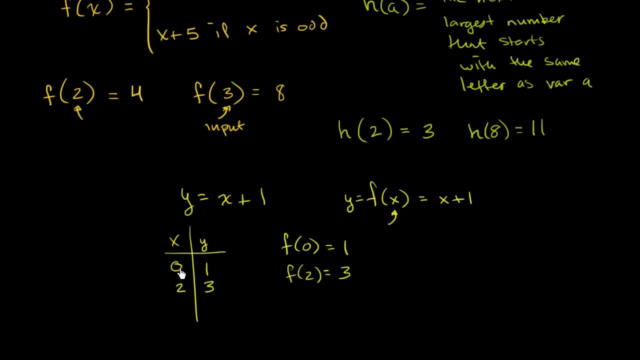 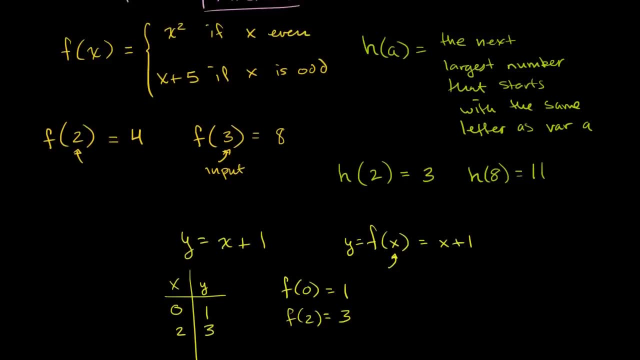 and then it produces one more than it. So here, whatever the input is, the output is one more than that original function. Now I know what you're asking, All right. well, what is not a function, then? Well, remember, we said, a function is something that takes an input. 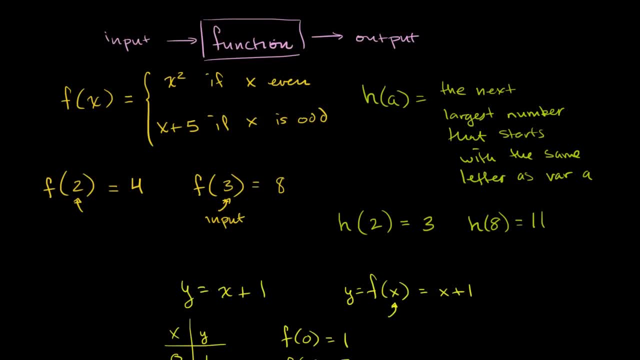 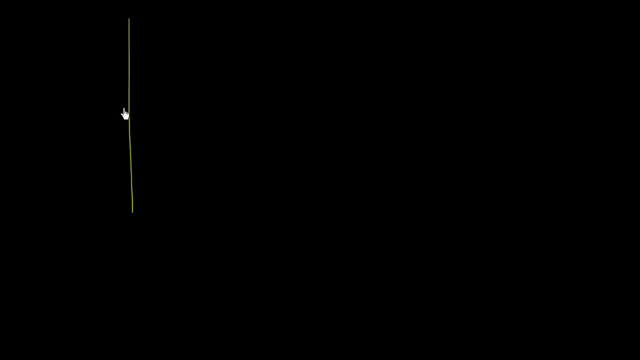 and produces only one possible output for that given input. So, for example, something like- and let me look at a visual way of thinking about a function this time I should say: So let's say that's our y-axis and this right over here is our x-axis. 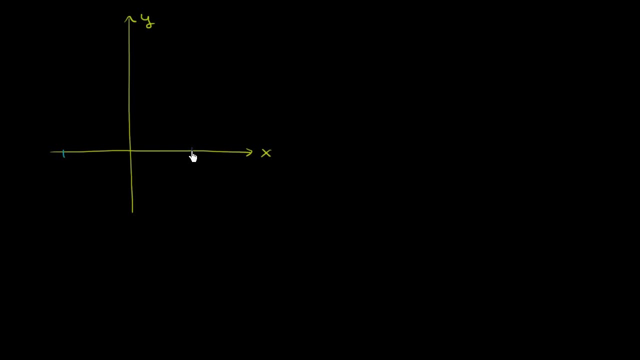 And let me draw a circle here that has radius 2. So it's a circle of radius 2.. This is negative, 2. This is positive, 2. This is negative, 2. So my circle, it's centered at the origin. 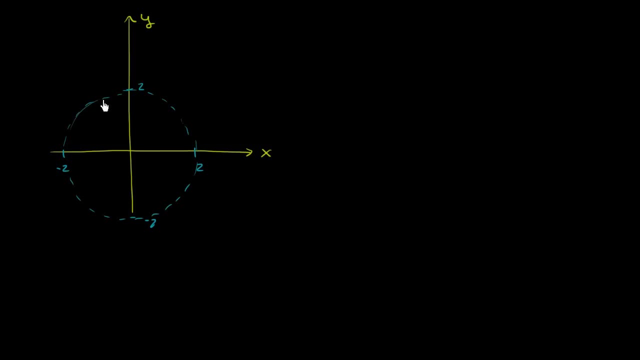 It has radius 2, so that's my best attempt at drawing the circle. Let me fill it in. So this is a circle. The equation of a circle, of this circle, is going to be: x squared plus y squared is equal to the radius squared. 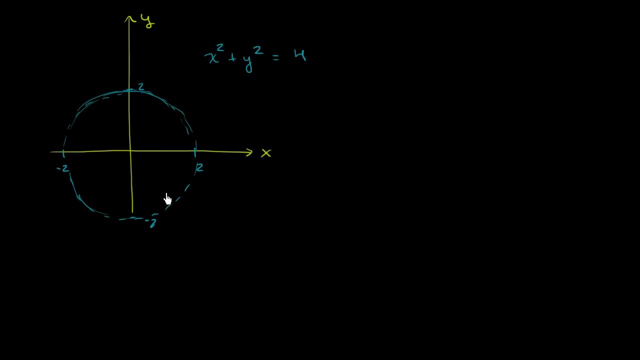 is equal to 2 squared, or it's equal to 4.. So the question is: is this relationship between x and y? here I've expressed it as equation, here I've visually drawn all of the x's and y's that satisfy this equation. 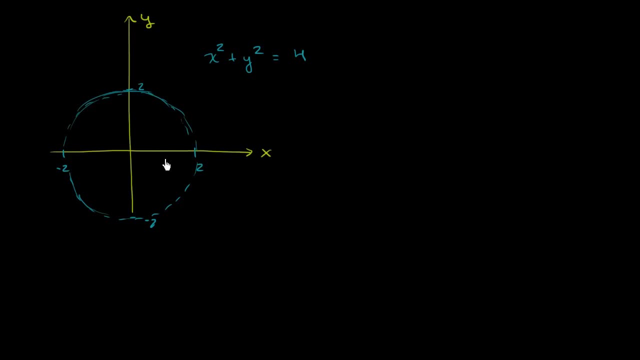 is this relationship between x and y a function? And we can see visually that it's not going to be a function. You pick a given x. Let's say x is equal to 1.. Let's say x is equal to 1.. 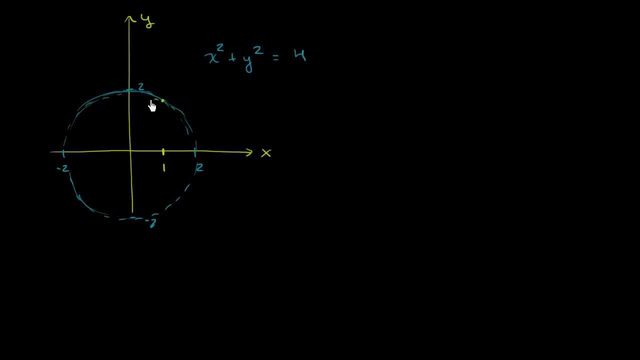 There's two possible y's that are associated with it- This y up here and this y down here- And we can even solve for that by looking at the equation: When x is equal to 1, we get 1 squared plus y squared is equal to 4..